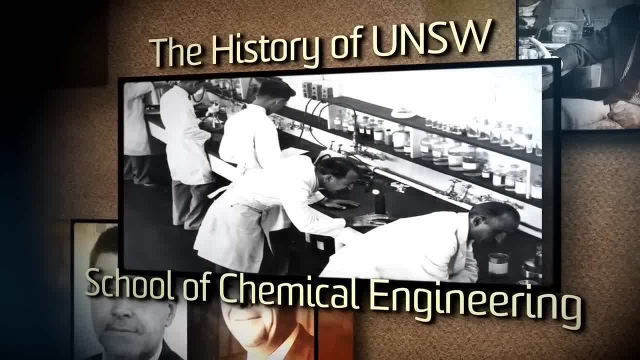 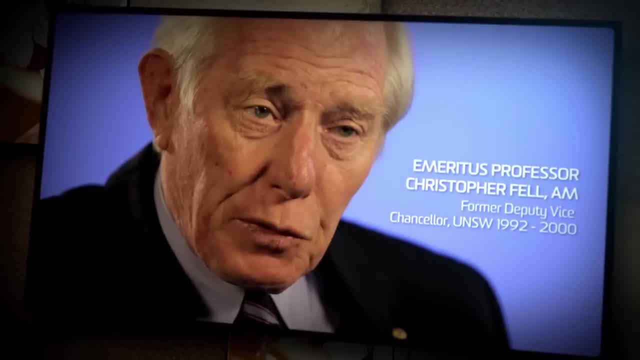 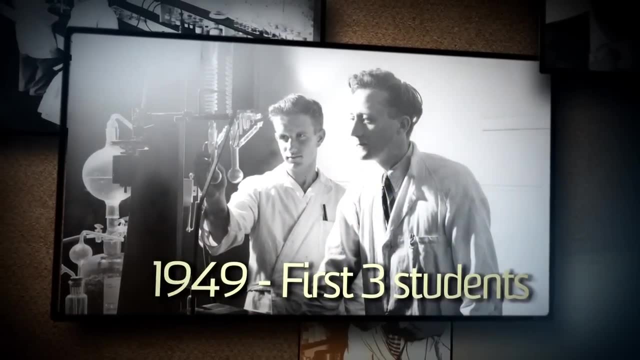 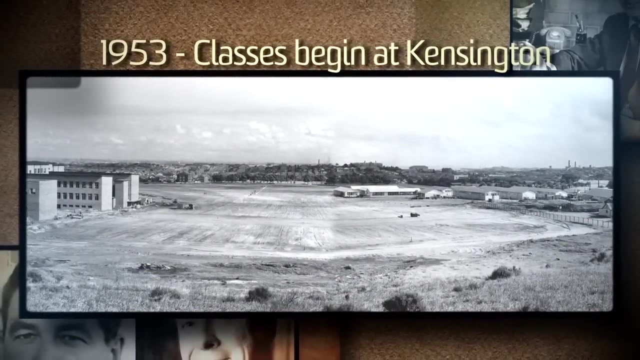 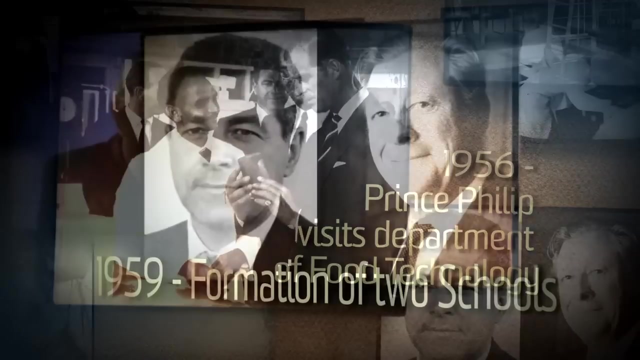 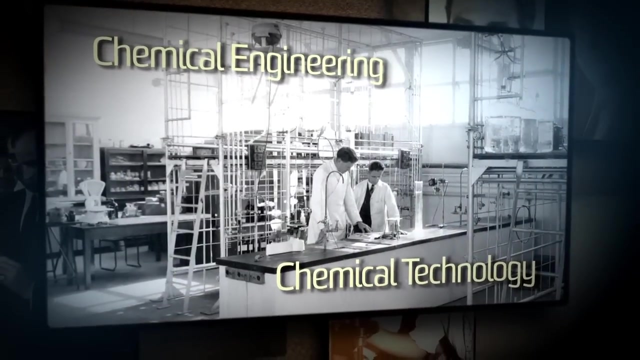 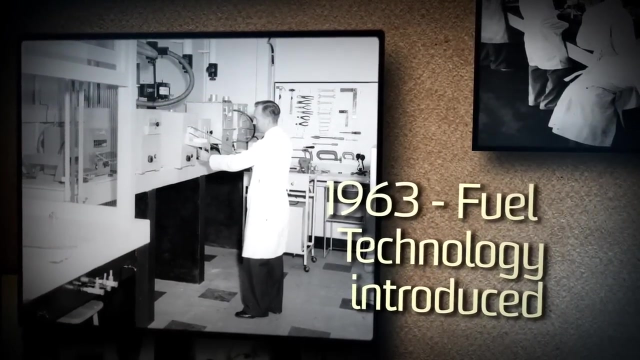 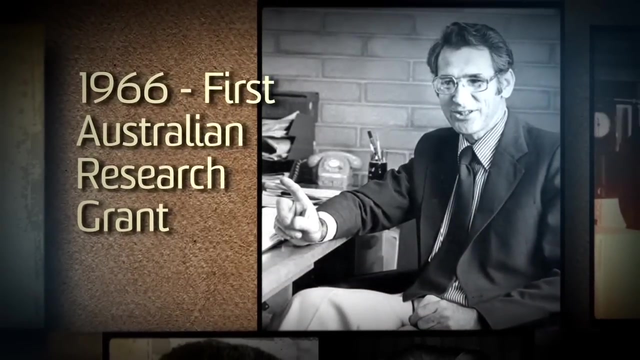 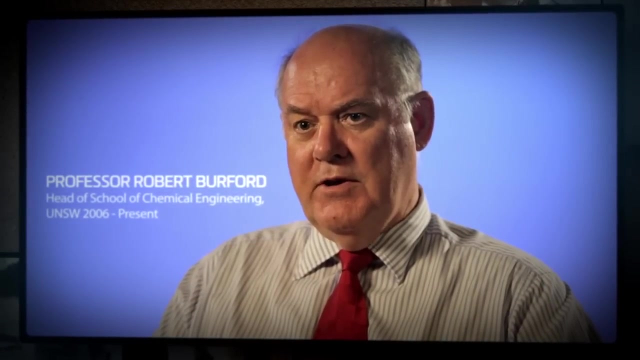 The school came from very humble beginnings to fairly quickly rise up to be a formidable presence nationally. We've been very lucky, I think, over the decades, to have what we call giants And for us, in succession, to stand on their shoulders and to become famous across the. 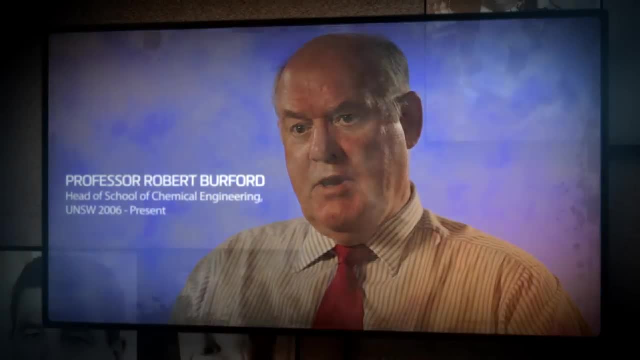 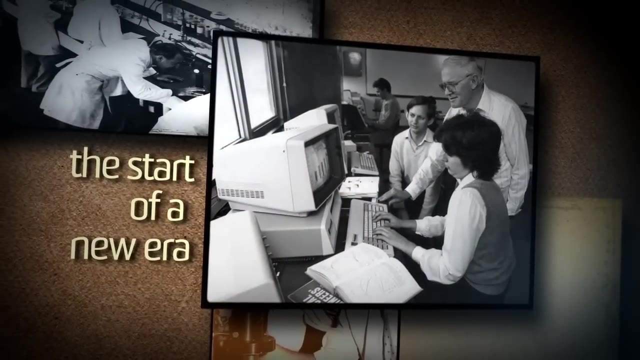 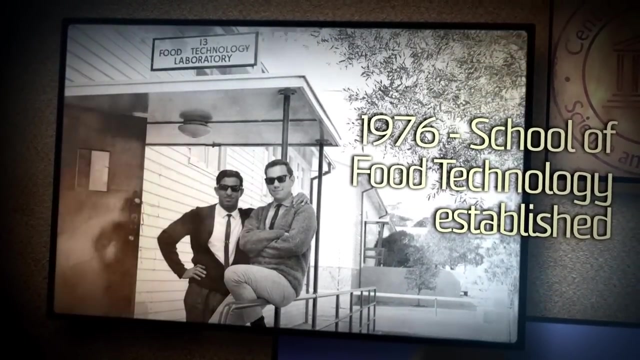 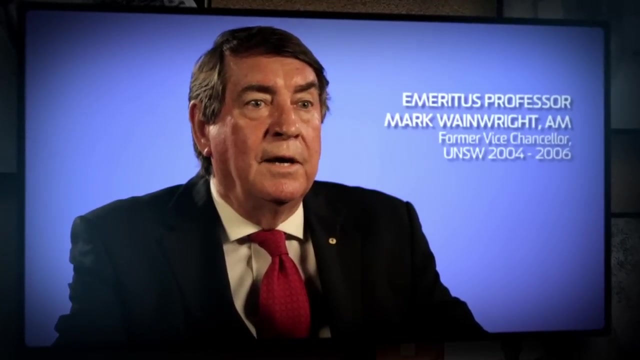 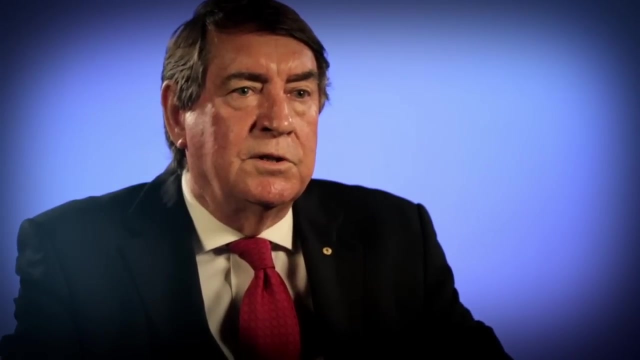 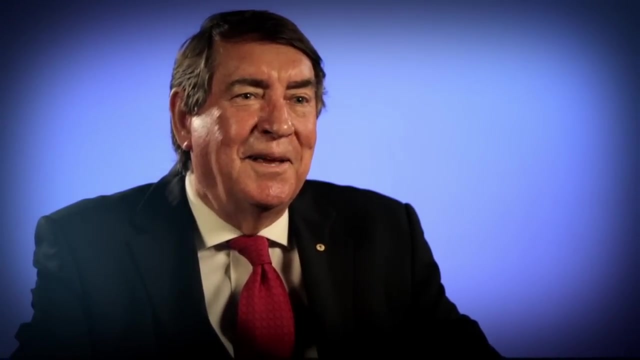 world. So we have a global reputation which continues today. The move went very amicably, It went very successfully and it brought to the Faculty of Engineering this huge research culture that both David Trim and Chris Fell- and perhaps I could say a little- brought. 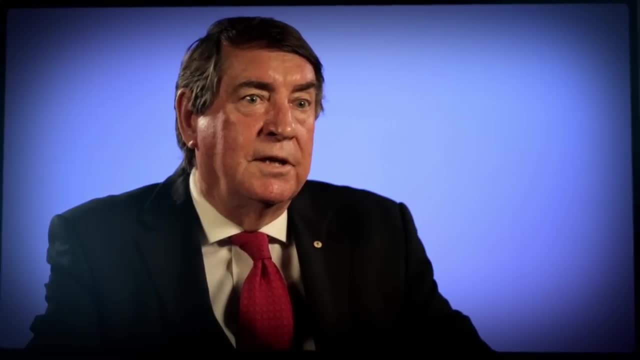 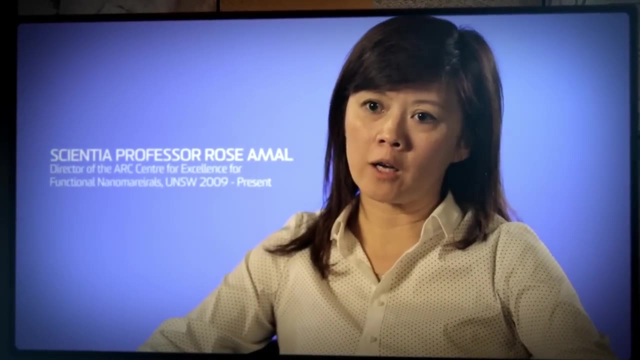 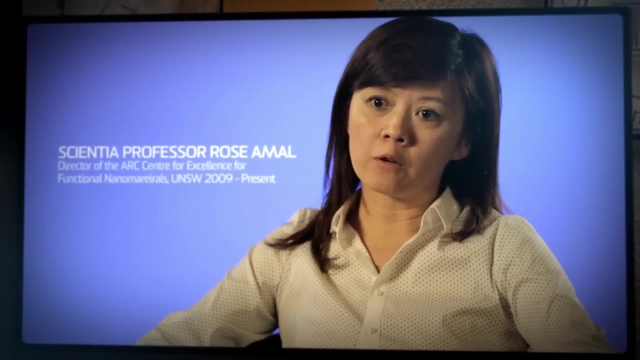 to the University in research. in the School of Chemical Engineering and Industrial Chemistry, David was my lecturer. He was my head of school and my colleague, and he was also a great friend. Most of us, including myself, would not be where we are now if it's not because of his. 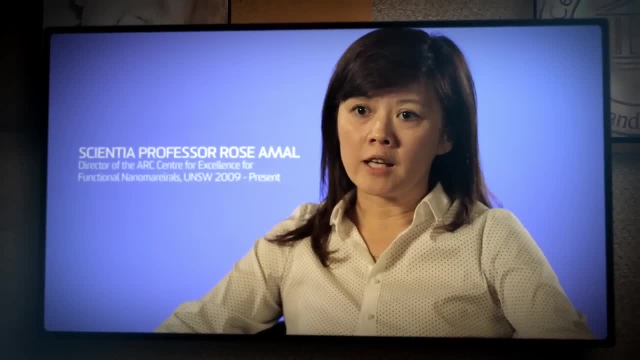 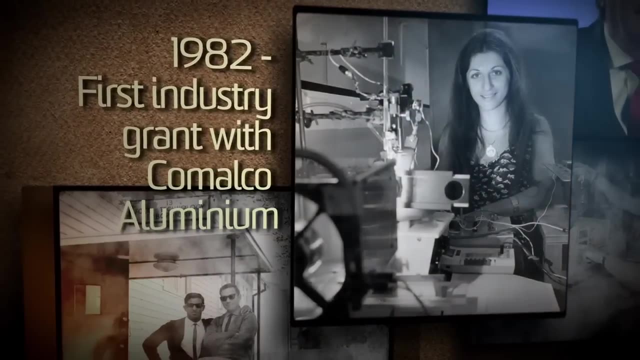 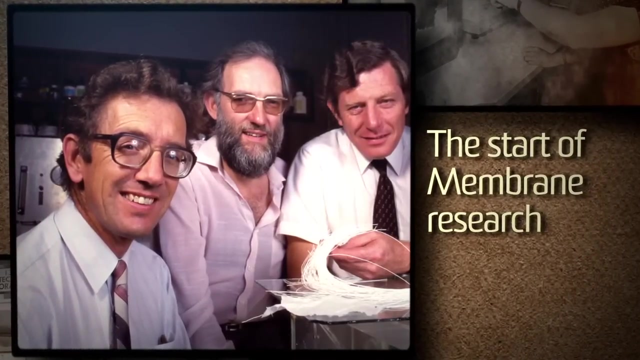 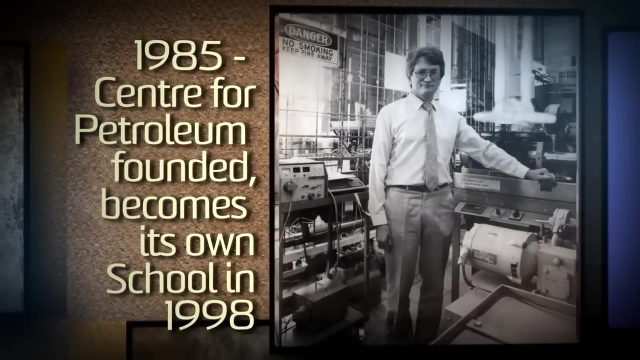 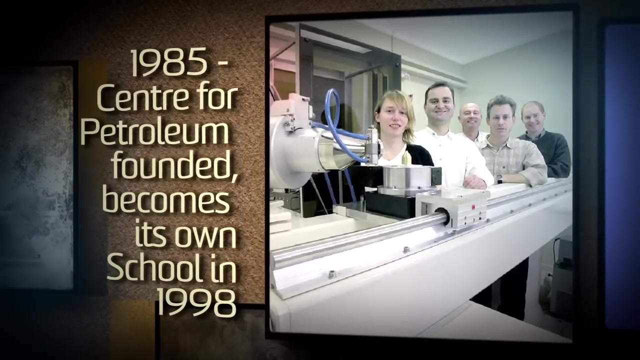 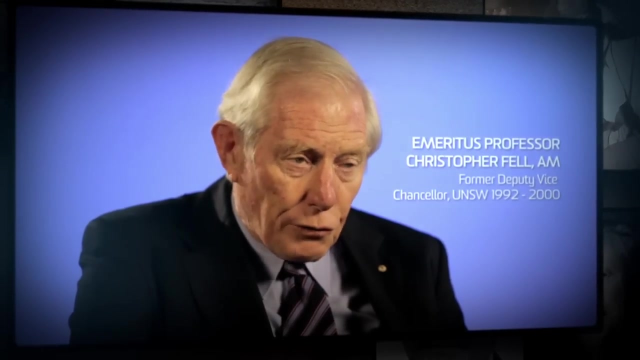 support and his guidance And I believe he had led and shaped the school to become one of the most prestigious schools in the country. ‑‑. Australia's largest company started to sending us, Sending Us- their cadets. So for a long time we had cadets sponsored by BHP, CSI and others.